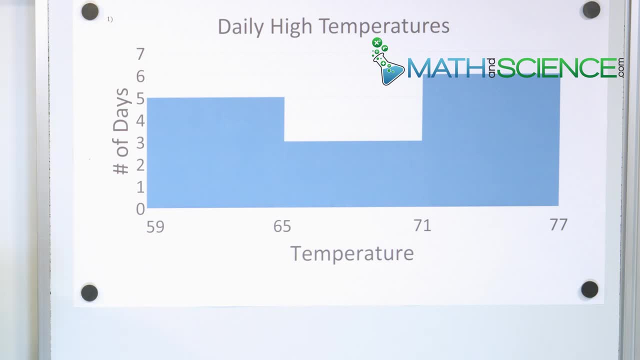 of a histogram. all right, Now I'm going to tell you right now that a histogram is essentially a bar chart. So if you have an idea of what a bar chart looks like, you know the vertical bars that go up. that's basically what a histogram is. There are a couple of differences, but ultimately, 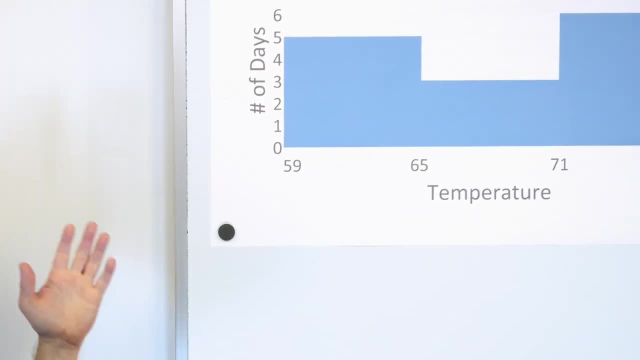 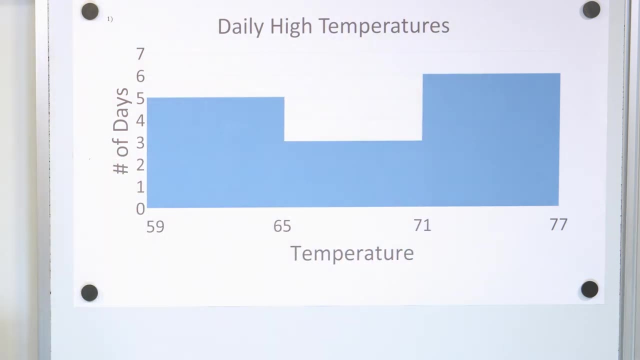 it looks just like a bar chart, with a couple of little differences there. What are the differences? Well, first of all, let's take a look at this one. This is a histogram of the daily high temperatures in a region, And so the way it is set up is on this axis, it's the number of days. 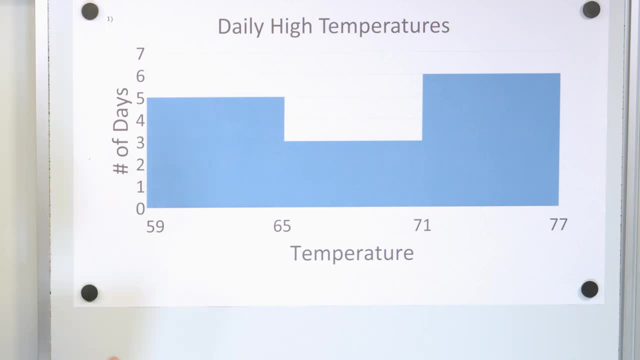 and on this axis it's the temperature ranges. Now this histogram. you know, in a bar chart, when you compare it, a bar chart with a histogram, there's two main things that are different In a bar chart. usually the bars have spaces between the bars. 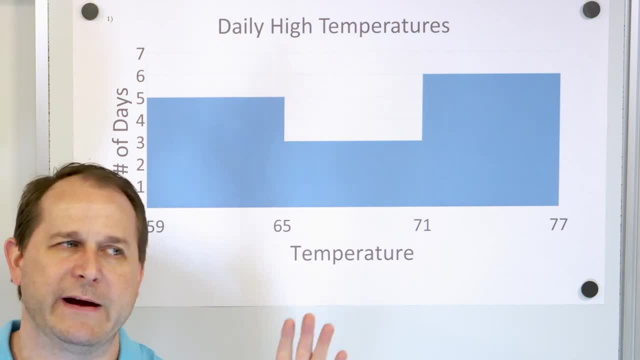 You notice that there's really no space between these bars. okay, So histograms, everything's crammed together. Secondly, in a bar chart along the bottom right here usually there are words or categories, Like a bar chart might be how many people like a favorite color could be on the. 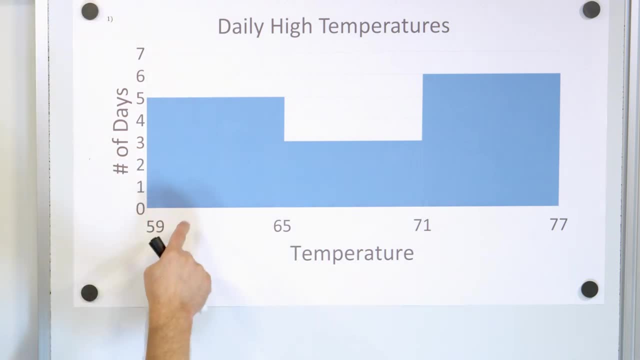 bottom and how many people like that color across the top. So this bar chart, if it were a bar chart, might be the color red, Here the color blue, Here the color green, And then here we're measuring how many people like red, blue and green. 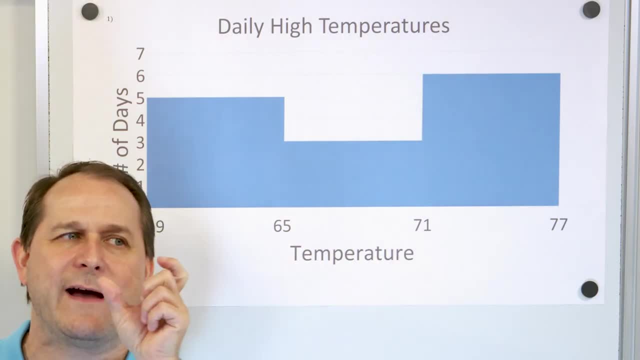 So for a bar chart, along the bottom usually we don't have numbers, we have words Like green, blue, yellow or who likes spaghetti versus soup versus steak- Words on the bottom. So two main differences between a histogram and a bar chart. For a bar chart, we have words along the bottom. 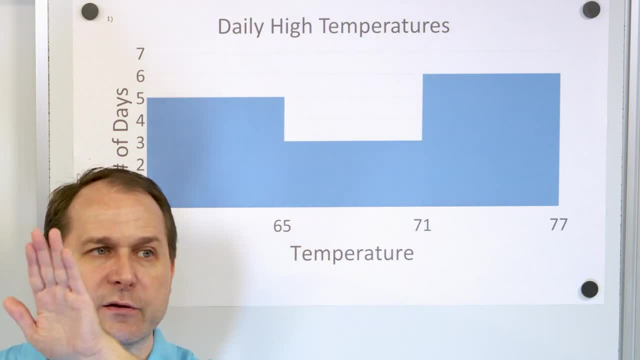 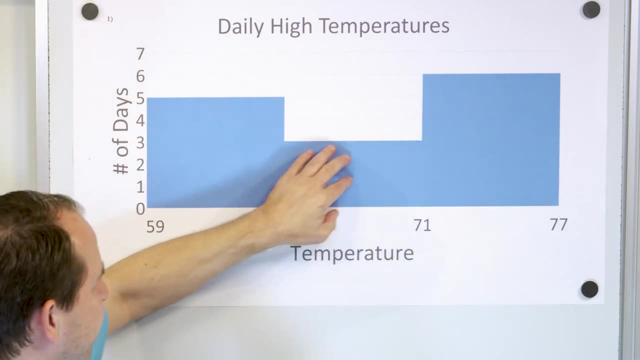 usually- and the bars are separated- The little things that go up the skyscrapers- they're separated with little spaces In a histogram. the bars are essentially connected together. There's really no space between them And along the bottom we have numbers. I'm going 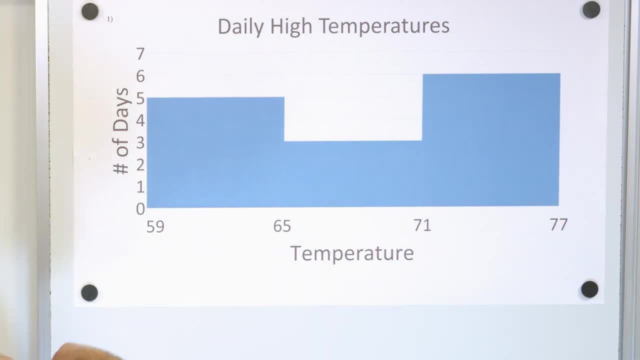 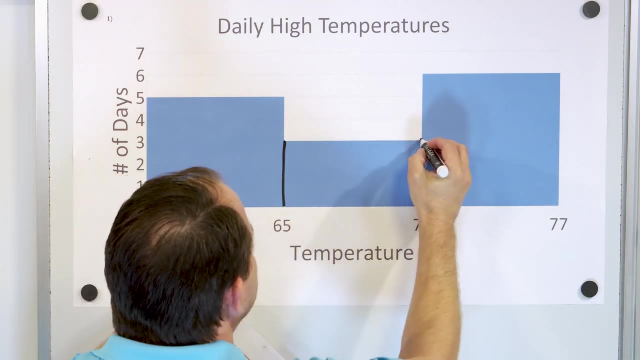 to talk more about the numbers in a second, Before I go any further, though, even though there's no space between them, it is perfectly fine for you to, either by hand or, depending on what you're using, your computer might draw little lines between the regions here. There's not supposed. 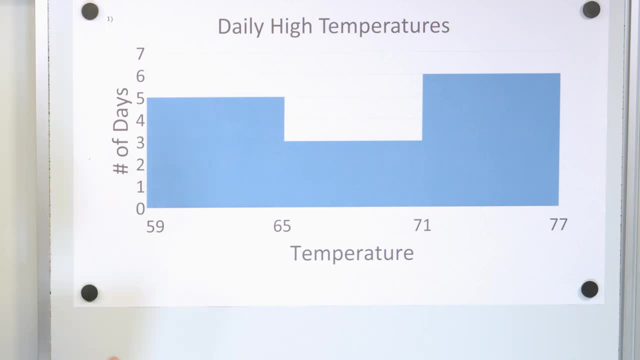 and on this axis it's the temperature ranges. Now this histogram. you know, in a bar chart, when you compare it, a bar chart with a histogram, there's two main things that are different In a bar chart. usually the bars have spaces between the bars. 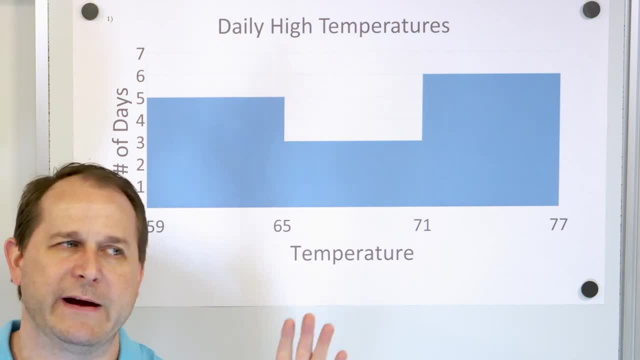 You notice that there's really no space between these bars. okay, So histograms, everything's crammed together. Secondly, in a bar chart along the bottom right here usually there are words or categories, Like a bar chart might be how many people like a favorite color could be on the. 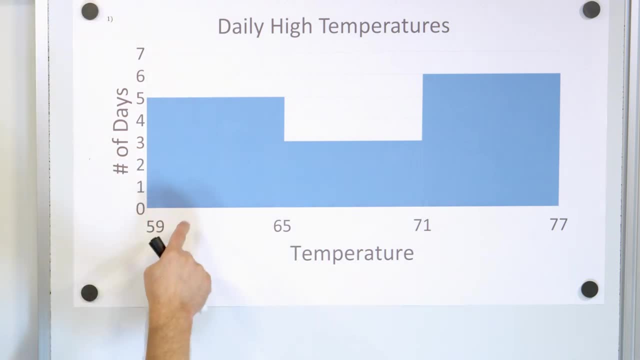 bottom and how many people like that color across the top. So this bar chart, if it were a bar chart, might be the color red, Here the color blue, Here the color green, And then here we're measuring how many people like red, blue and green. 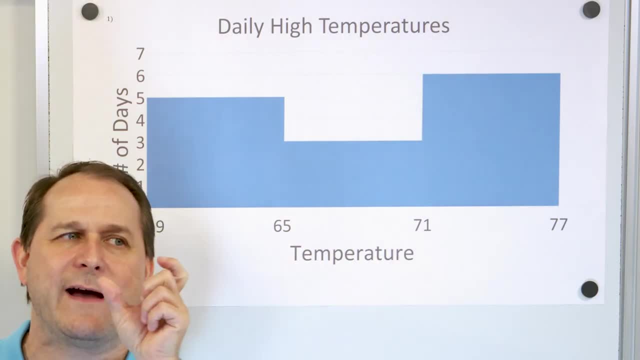 So for a bar chart, along the bottom usually we don't have numbers, we have words Like green, blue, yellow or who likes spaghetti versus soup versus steak- Words on the bottom. So two main differences between a histogram and a bar chart. For a bar chart, we have words along the bottom. 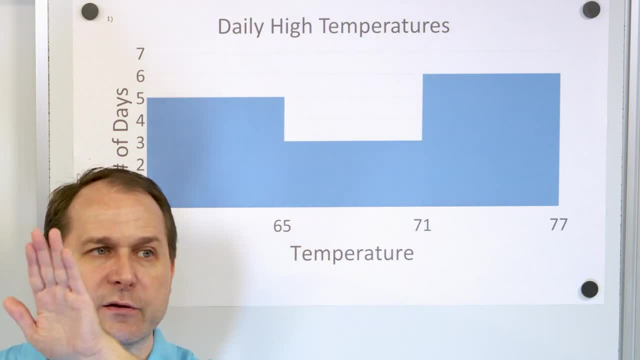 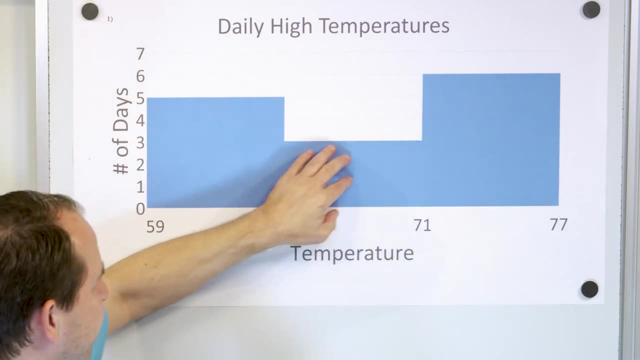 usually- and the bars are separated- The little things that go up the skyscrapers- they're separated with little spaces In a histogram. the bars are essentially connected together. There's really no space between them And along the bottom we have numbers. I'm going 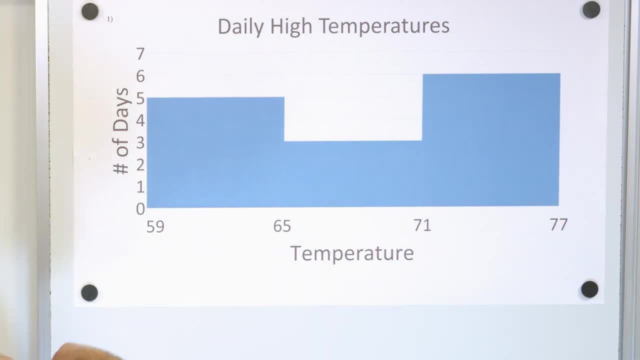 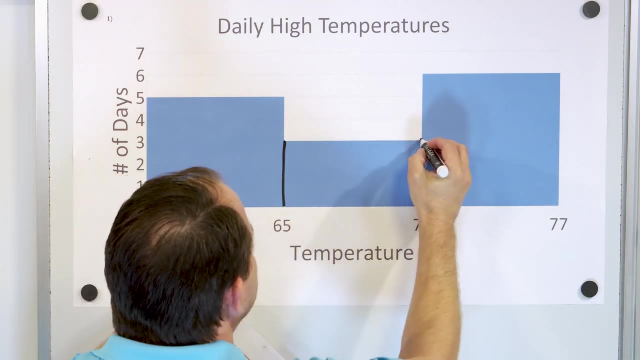 to talk more about the numbers in a second, Before I go any further, though, even though there's no space between them, it is perfectly fine for you to, either by hand or, depending on what you're using, your computer might draw little lines between the regions here. There's not supposed. 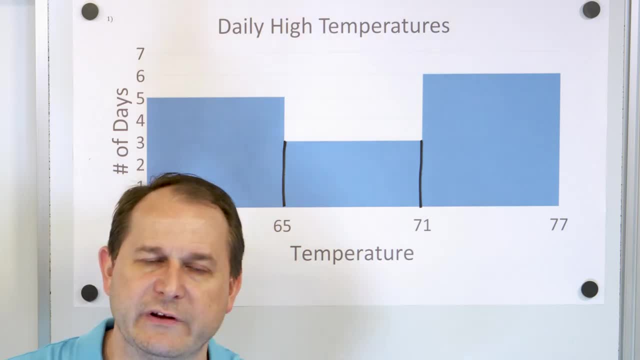 to be any space between the bars, but there can certainly be lines so that you can read the thing a little bit easier. So that's why I say it's like a bar chart. This one goes up to five days. this one goes up to three days. this one, as you read it off, goes up to six days. Now let's take 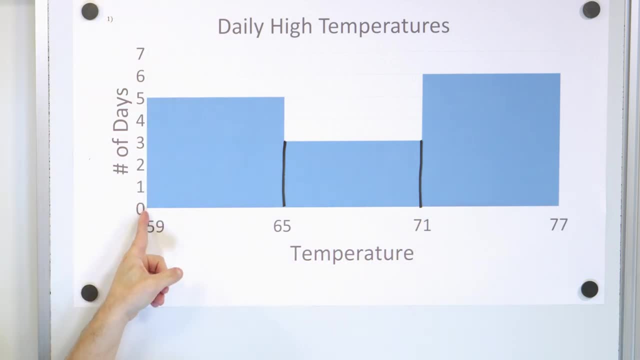 a look at the numbers that are along the bottom, Notice that the numbers are only on the kind of the edges between where one bar starts and the other one goes. So we have to look at the numbers. Here we have 59 degrees to 65 degrees and the difference here between 65 and 59 is six degrees. 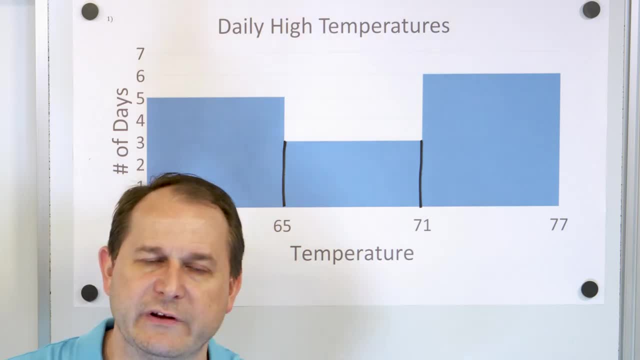 to be any space between the bars, but there can certainly be lines so that you can read the thing a little bit easier. So that's why I say it's like a bar chart. This one goes up to five days. this one goes up to three days. this one, as you read it off, goes up to six days. Now let's take 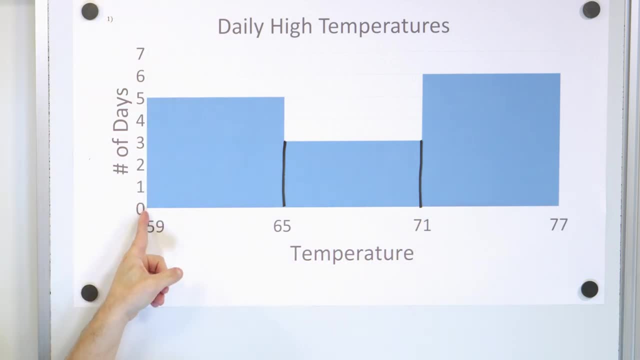 a look at the numbers that are along the bottom, Notice that the numbers are only on the kind of the edges between where one bar starts and the other one goes. So we have to look at the numbers. Here we have 59 degrees to 65 degrees and the difference here between 65 and 59 is six degrees. 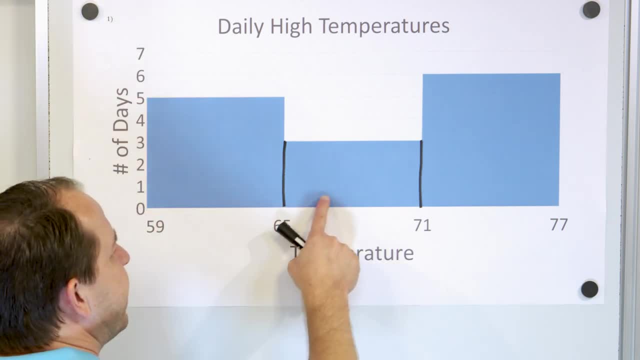 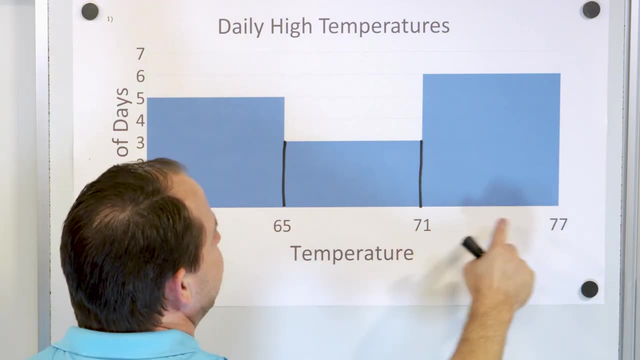 So the width of this bar is six degrees right. Then we have 65 to 71 degrees- Again six degrees width. And here we have 71 to 77, again six degrees width. So for a histogram usually what? 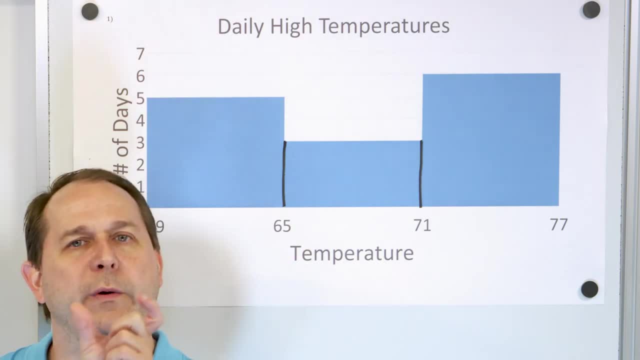 you want to do. you want to have the ranges of the numbers on the bottom always be the same width. You can think of it like buckets. You have three different buckets, you know. on the bottom It's just sitting outside right. One bucket is asking you: did the temperature range go from 59? 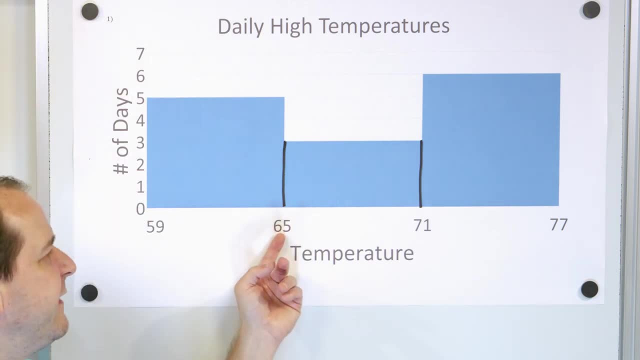 to 65 degrees And the next bucket says is the temperature 65 to 71 degrees. And the third bucket that you have on the ground you label it going from 71 to 77 degrees And then you measure the temperature every single day. If the temperature that day falls between 59 and 65, you put a piece. 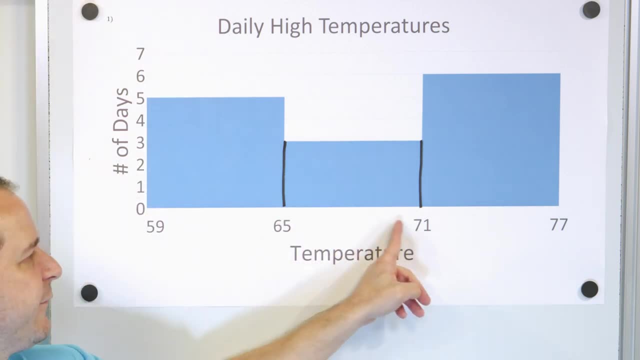 of paper in that bucket, the first bucket, But if the temperature falls in this range, you put something in the second bucket And then, of course, if it falls in this third range, you put it in the third bucket. At the end of your study you count how many. 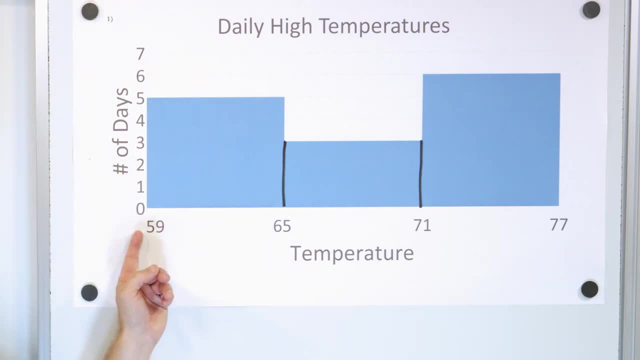 how many entries you have in bucket number one, So the number of days that the temperature really did range from 59 to 75 degrees, And then you put it in the second bucket, And then you put it in the third bucket, And then you put it in the third bucket, And then you put it in the third bucket, And 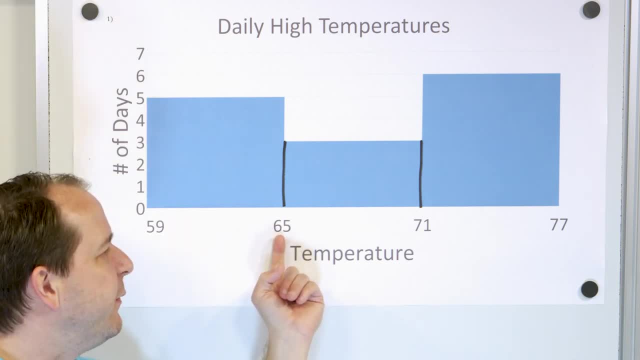 the number of days that it ranged from 59 to 65 was five days. The number of days between 65 and 71 degrees was actually three, And the number of days between 71 and 77 was actually six days. So bottom line is it looks like a bar chart but we call it a histogram, because a histogram means 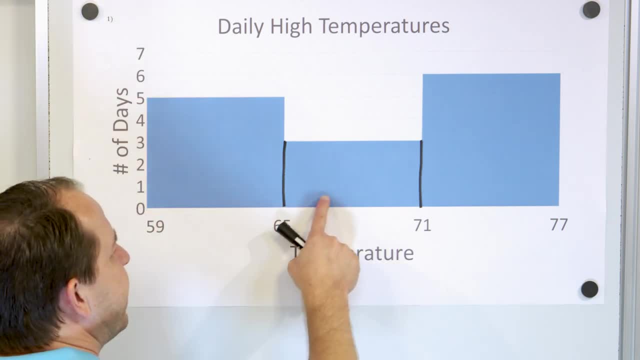 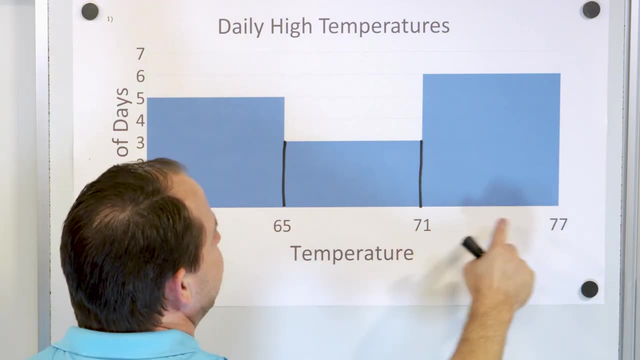 So the width of this bar is six degrees right. Then we have 65 to 71 degrees- Again six degrees width. And here we have 71 to 77, again six degrees width. So for a histogram usually what? 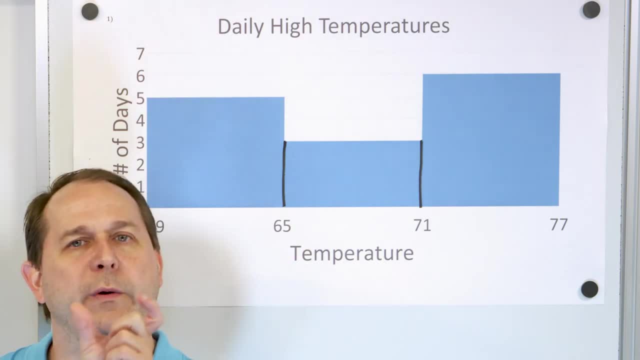 you want to do. you want to have the ranges of the numbers on the bottom always be the same width. You can think of it like buckets. You have three different buckets, you know. on the bottom It's just sitting outside right. One bucket is asking you: did the temperature range go from 59? 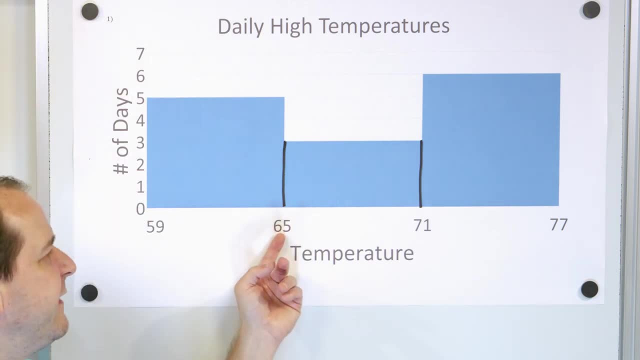 to 65 degrees And the next bucket says is the temperature 65 to 71 degrees. And the third bucket that you have on the ground you label it going from 71 to 77 degrees And then you measure the temperature every single day. If the temperature that day falls between 59 and 65, you put a piece. 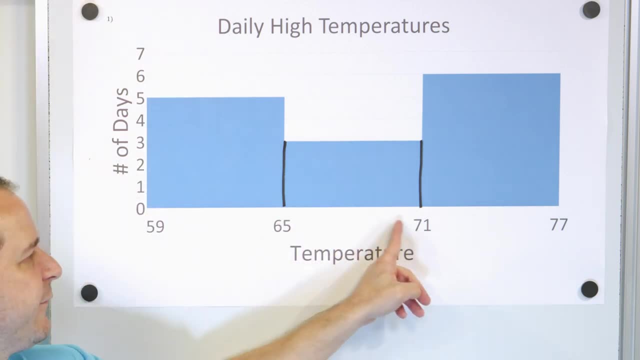 of paper in that bucket, the first bucket, But if the temperature falls in this range, you put something in the second bucket And then, of course, if it falls in this third range, you put it in the third bucket. At the end of your study you count how many. 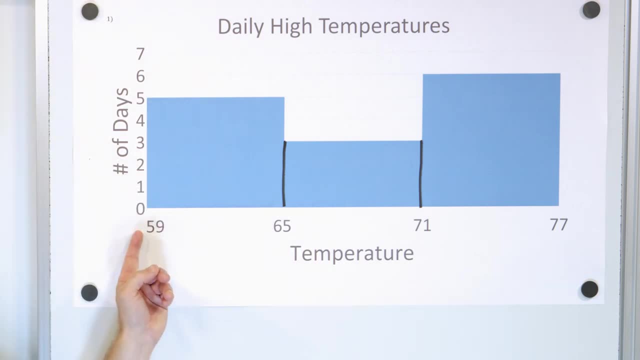 how many entries you have in bucket number one, So the number of days that the temperature really did range from 59 to 75 degrees, And then you put it in the second bucket, And then you put it in the third bucket, And then you put it in the third bucket, And then you put it in the third bucket. 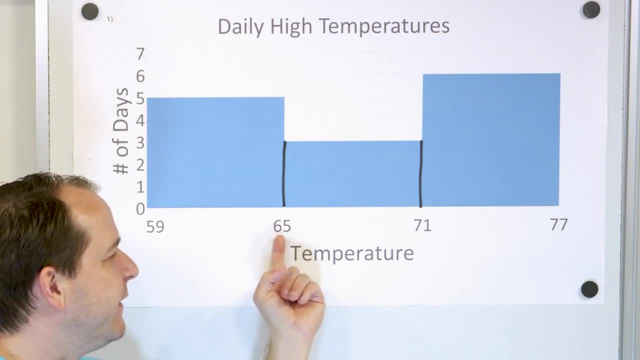 So the number of days that the temperature really did range from 59 to 65 was five days. The number of days between 65 and 71 degrees was actually three And the number of days between 71 and 77 was actually six days. So bottom line is it looks like a bar chart, but we call it a. 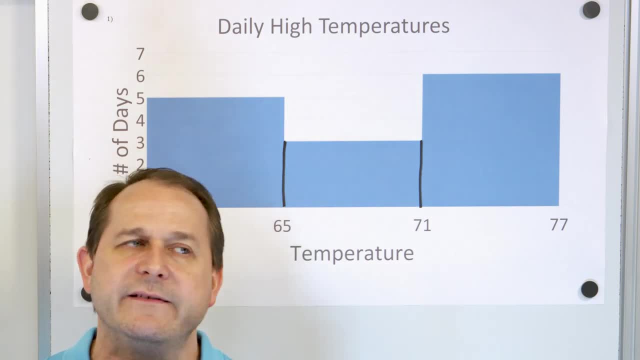 histogram, because a histogram means something special. It means that the labeling along the bottom are numbers. no, no colors or or words. it's numbers, And the numbers are only listed at the boundary of the different bars, And then you put it in the third bucket, And then you put it in. 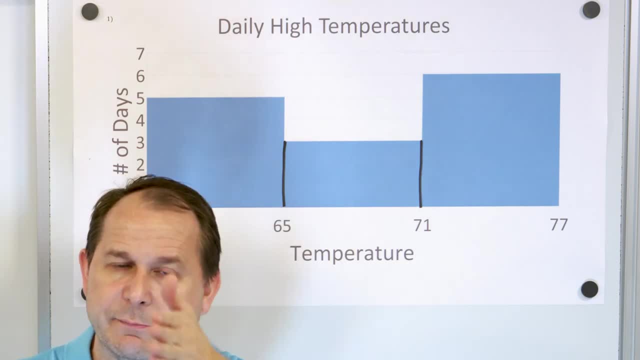 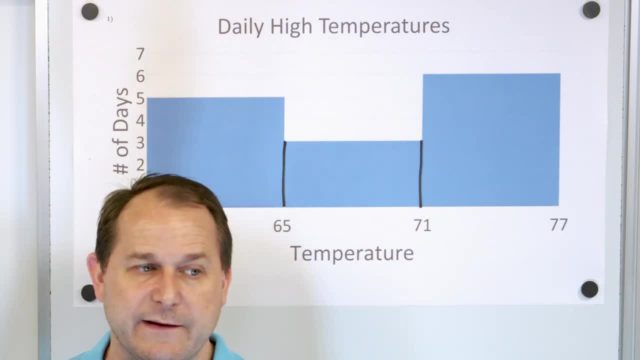 when you subtract, has should always be the same width for a histogram. The different buckets are the same width, essentially. And then, on this axis here, what you're measuring is: how many times did this- uh, whatever it is you're talking about- happen? How many times was the temperature in? 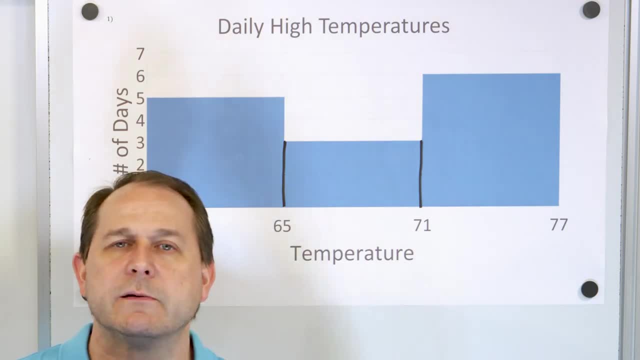 something special. It means that the labeling along the bottom are numbers. No, no colors or or words. it's numbers And the numbers are only listed at the boundary of the different bar and the bars are touching. there you can have lines, but they're always touching. 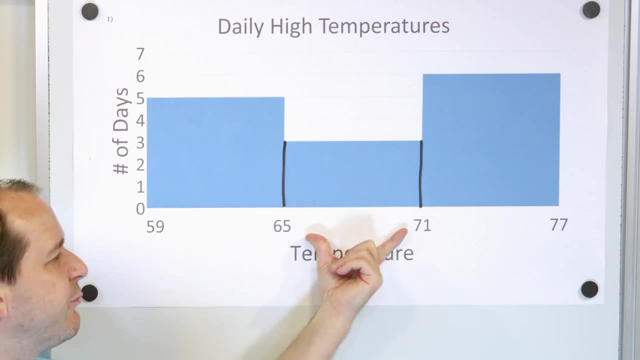 and the width in the numbers when you subtract has should always be the same width for a histogram. the different buckets are the same width essentially. and then, on this axis here, what you're measuring is: how many times did this, whatever it is you're talking about- happen? how many times was the? 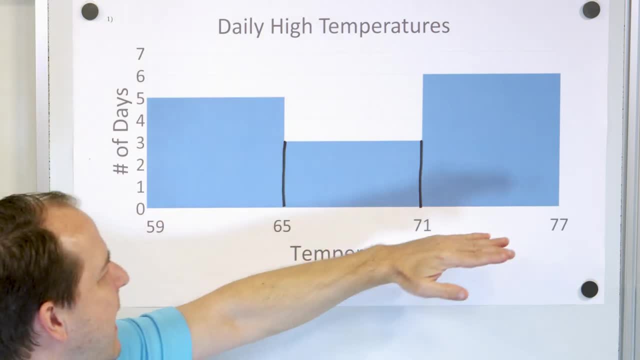 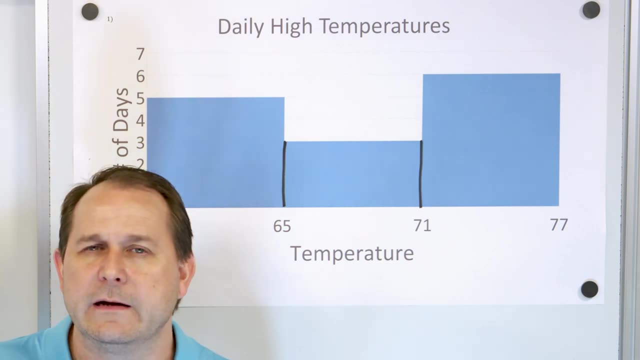 temperature in this range, how many times was the temperature in this range? how many times was the temperature in this range? so that is what a histogram is you're measuring, kind of the frequency, the frequency which is how many times something happens, and the different ranges have to all be the same width in. 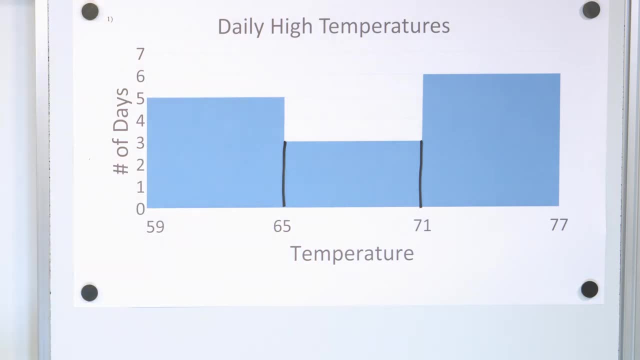 order for it to make sense. all right, so let's answer number one and let's see how we can use a histogram to answer some really basic questions. all right, question number one: for how many days was the temperature between 65 and 71 degrees? so how many days was the temperature between 65 and 71 degrees so? 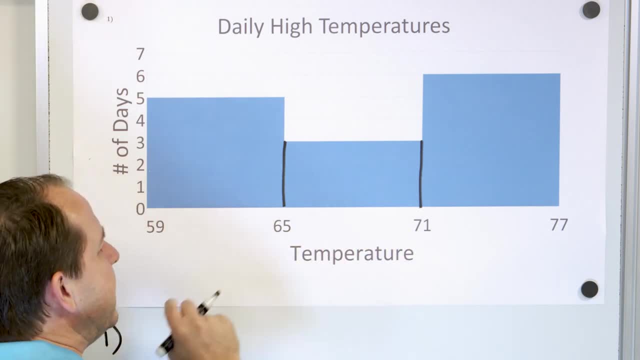 you look here and you have a bucket here. we call it a bin and the bin here is listed from 65 degrees to 71 degrees. so in this window from 65 to 71, we can see that only three days had that that range here. right, maybe it was 66. 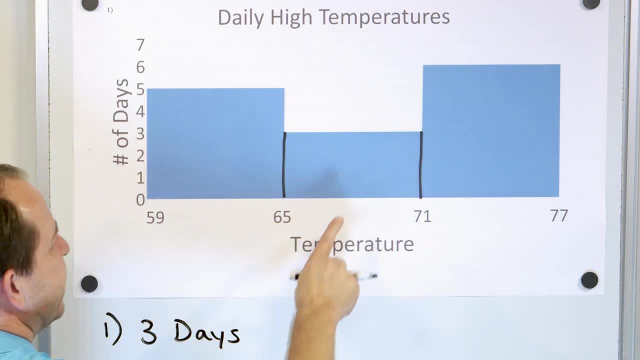 degrees one day, maybe it was seven degrees another day, maybe it was 69 degrees another day, but only three days was it in this range at all? so we say three days. question number two: for how many days was the temperature 65 degrees or above? how many days was the temperature? 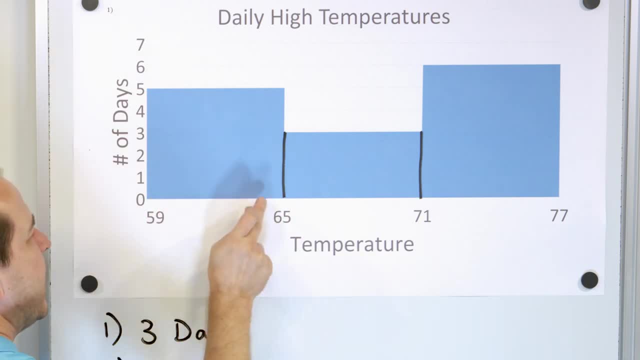 65 degrees or above. Well, you can see we have a bend from 59 to 65, but if we're looking at days when temperature was 65 degrees or above, it's going to go from here all the way to the end of. 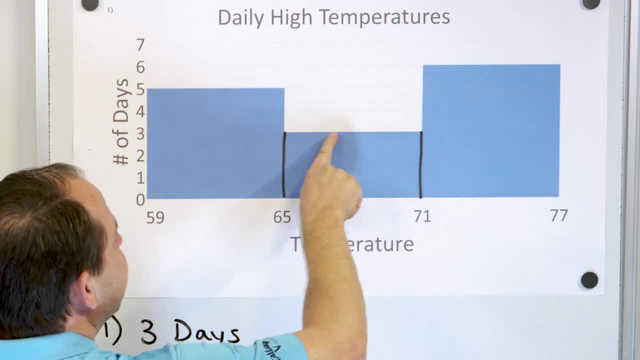 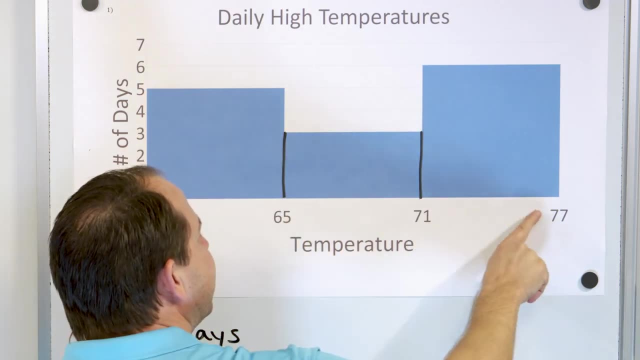 the chart to 77. We know that three days we had three days in this window to 71 degrees, but we also had six more days in the range of 71 to 77. So what we do is we take that three and we add it. 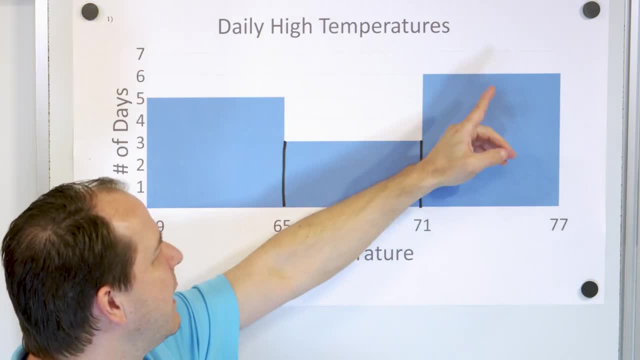 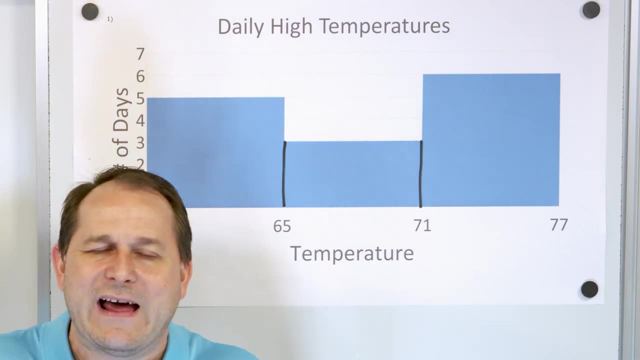 this range? How many times was the temperature in this range? How many times was the temperature in this range? So that is what a histogram is: You're measuring the temperature in this range And then kind of the frequency, which is how many times something happens and the different ranges have. 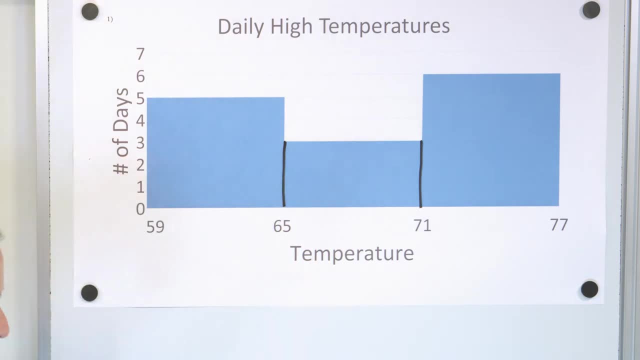 to all be the same width in order for it to make sense. All right, so let's answer number one and let's see how we can use a histogram to answer some really basic questions. All right, question number one: for how many days was the temperature between 65 and 71 degrees? So how many days was? 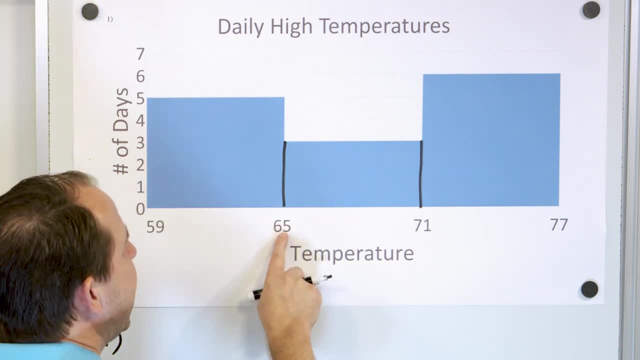 the temperature between 65 and 71 degrees. So you look here and you have a bucket here. we call it a bin and the bin here is listed from 65 degrees to 71 degrees. So in this window from 65 to 71, we 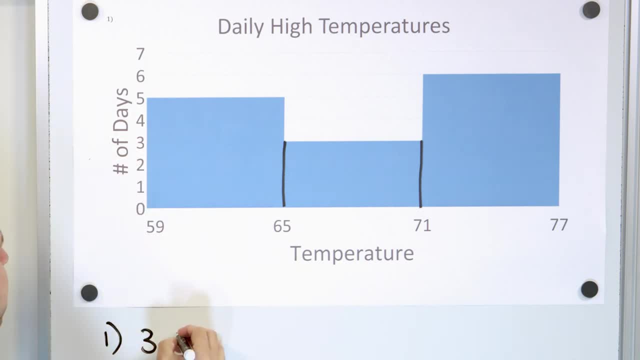 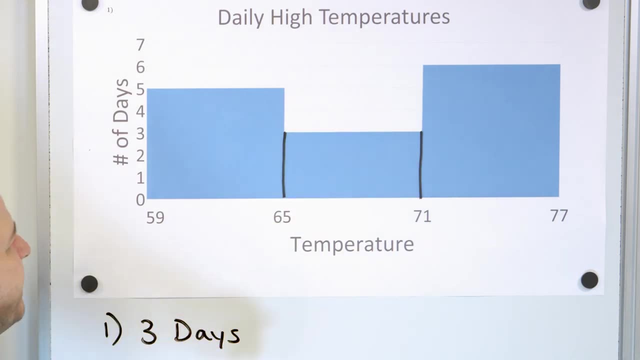 can see that only three days had that range here, right? Maybe it was 66 degrees one day, maybe it was seven degrees another day, maybe it was 69 degrees another day, but only three days was it in this range at all. So we say three days. Question number two: for how many days was the 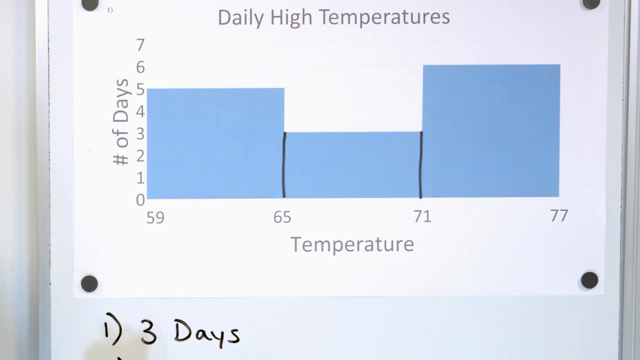 temperature 65 degrees or above. How many days was the temperature 65 degrees or above? Well, you can see we have a bin from 59 to 65. But if we're looking at days when temperature was 65 degrees or above, it's going to go from here. 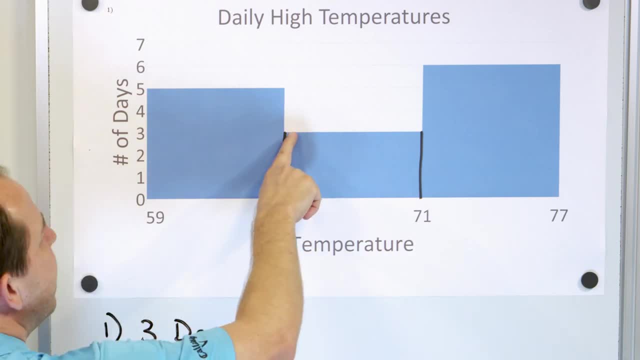 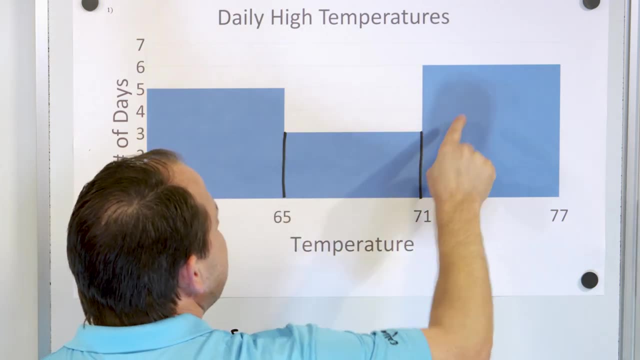 all the way to the end of the chart to 77. We know that three days we had three days in this window to 71 degrees, but we also had six more days in the range of 71 to 77. So what we do is we take that. 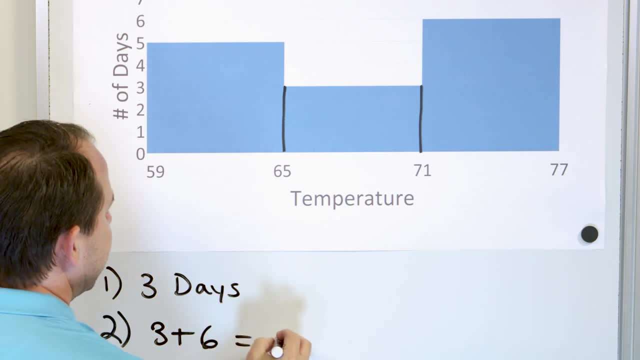 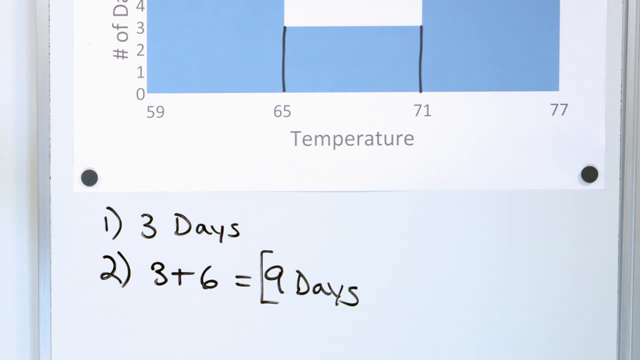 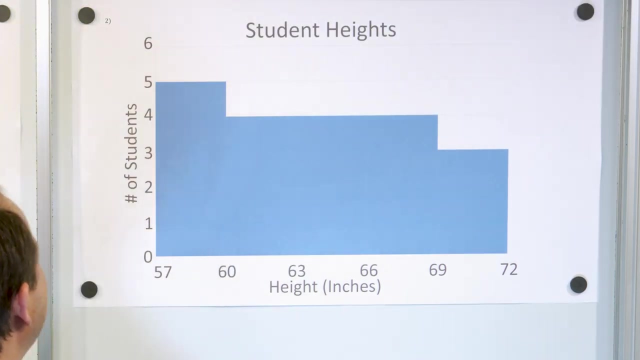 three and we add it to the six and that's nine days. So in nine days, was the temperature 65 degrees or above All? right, let's take a look at histogram number two. So here we have a histogram of the height of students, right? So we go and we line up. 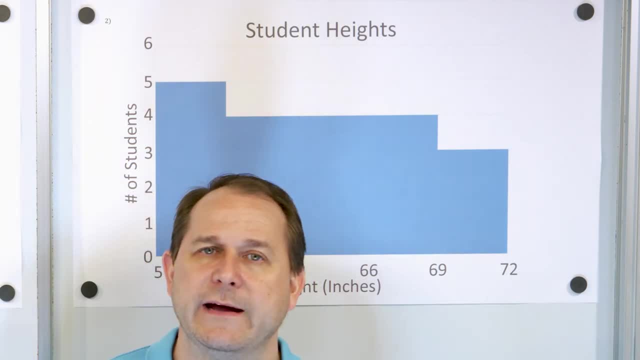 all of our students against the wall and we measure all of their heights right, And so we have to. we're not listing every single data point here. what we're doing is we're creating bins or buckets, And the width of the buckets: here we can see 57 to 60.. 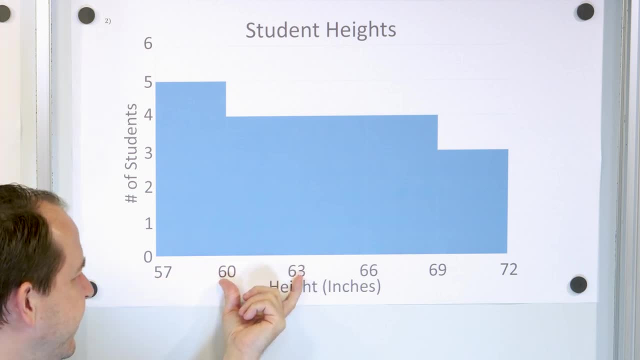 That is a width of three. 60 to 68,. that's a width of three. 63 to 66, that's a width of three. Here's another width of three. Here's another width of three. You see, for a histogram, the widths along the bottom have to be the same. 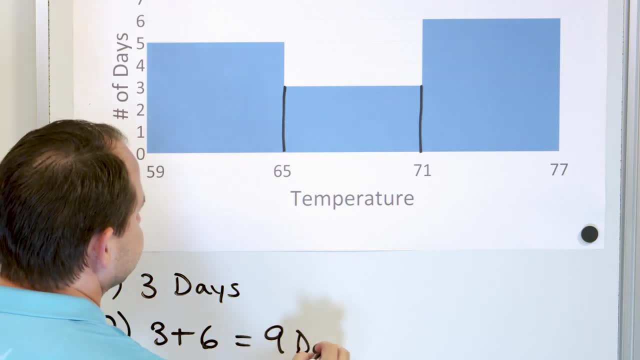 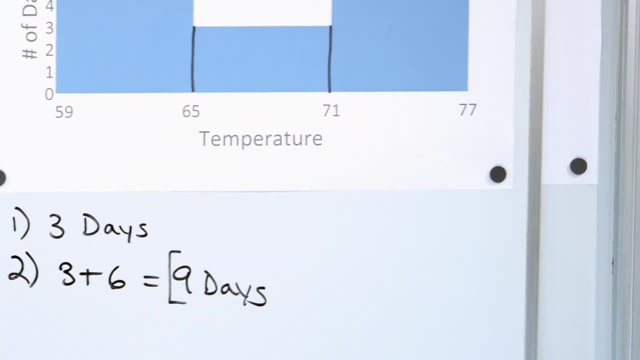 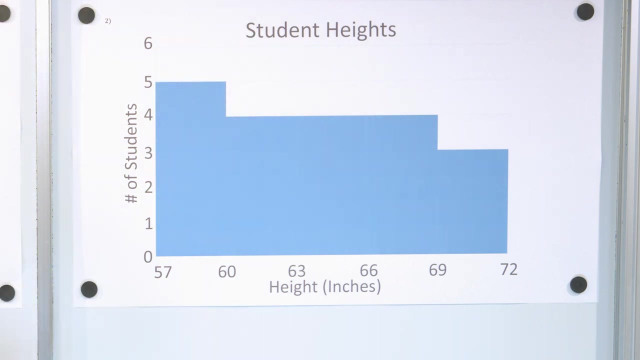 to the six, and that's nine days. So in nine days, was the temperature 65 degrees or above All? right, let's take a look at histogram number two. So here we have a histogram of the height of students, right? So we go and we line up all of our students against the wall and we measure. 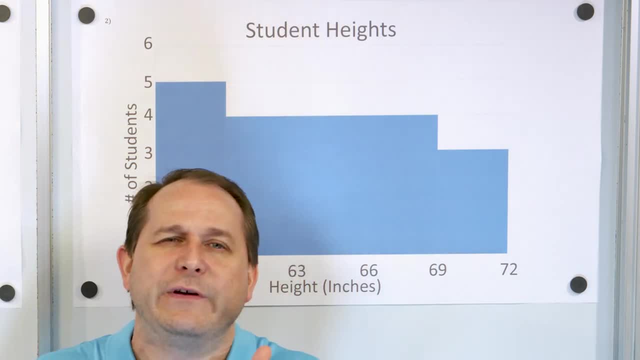 all of their heights, right, And so we have to. we're not listing every single data point here. What we're doing is we're creating bins or buckets, and the uh width of the buckets- here we can see 57 to 60.. Um, that is a width of three: 60 to 68.. That's a 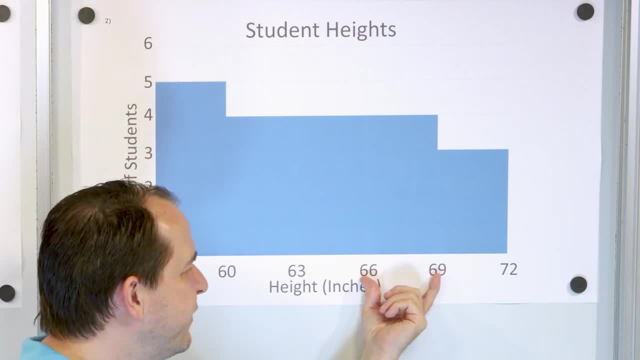 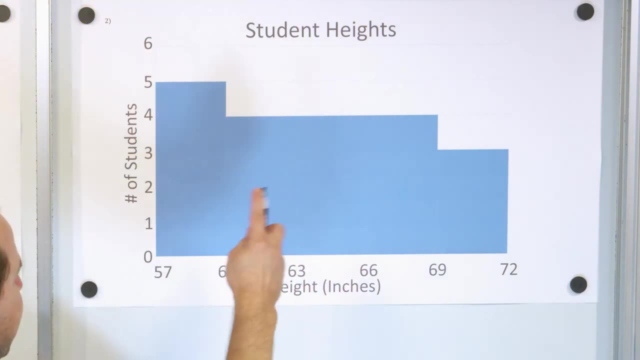 width of three: 63 to 66.. That's a width of three. Here's another width of three. Here's another width of three. You see, for a histogram the widths along the bottom have to be the same. Now, in my particular program I don't have any any. uh, everything's pushed together. 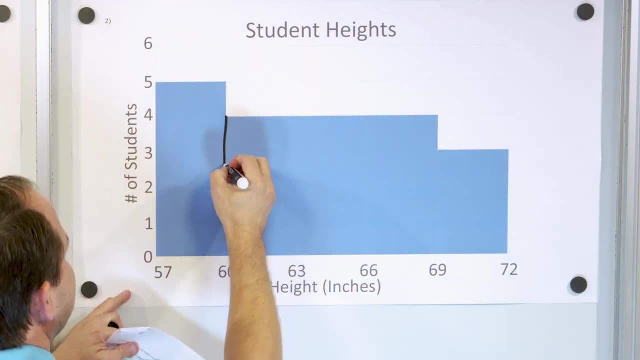 but I don't have any uh gaps So it's a little hard to read. So if you want to, you can draw lines. Uh, some people like to see these lines, Some people don't. you can do whatever you. 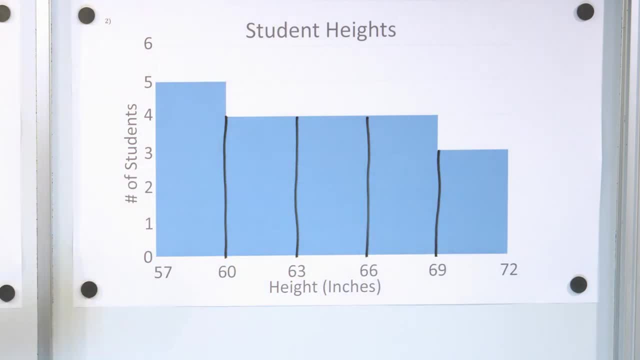 want to me. I'm not a real stickler, I just want you to be able to read the thing, but you should not have any gaps between them, All right. So the question is, how do we read this thing? So you could say, for instance, between 60 and 63 inches. right, We had four students in there Now. 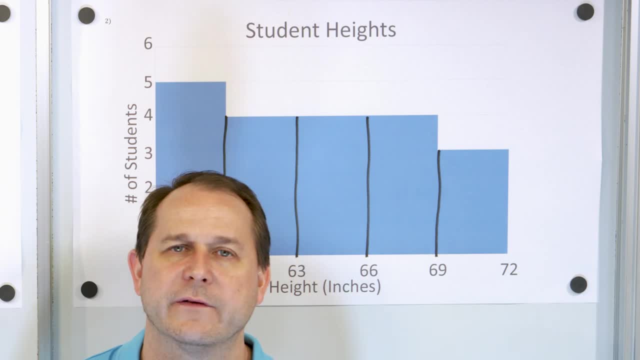 it doesn't tell me the actual heights of those four students. So a histogram is taking the data you have and it's presenting it to you without showing you every single data point. We are throwing some data away because we want to get an overall picture of what's happening And you can. 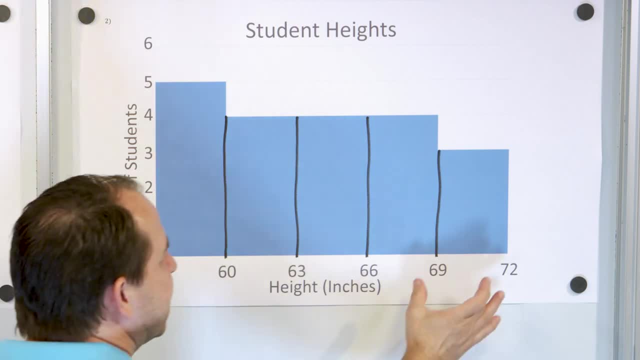 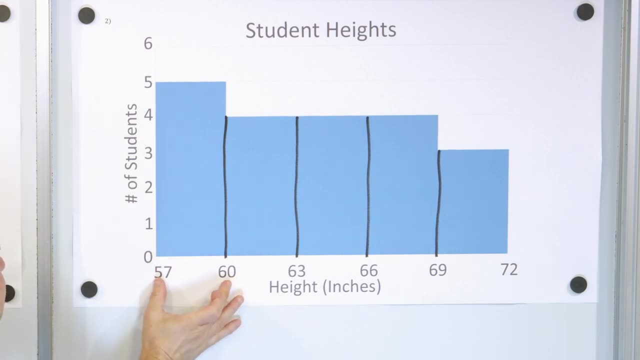 look at this and say, well, okay, I have most students down in this range and I have the least number of students over in this range. but we lose a little bit of the raw data because we only know, for instance, between here, between 57 and 60 inches, we had five students, but I don't know. 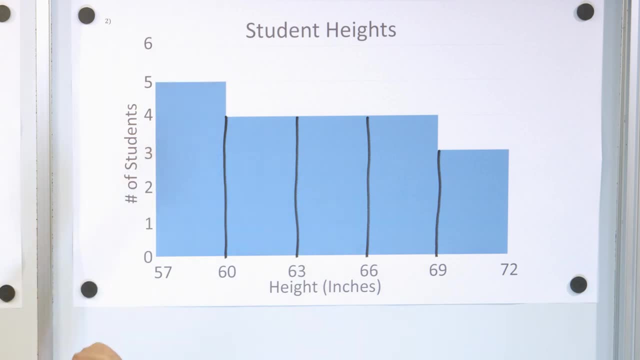 if they were 58 inches or 57 inches or 59. I don't really know. I just know I have five of them in this window. All right, Let's take a look at question number one. All right. Question number one says how many students are 66 inches or taller. How many students are 66 inches or? 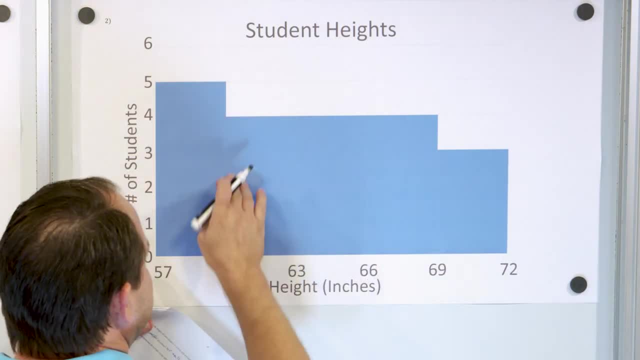 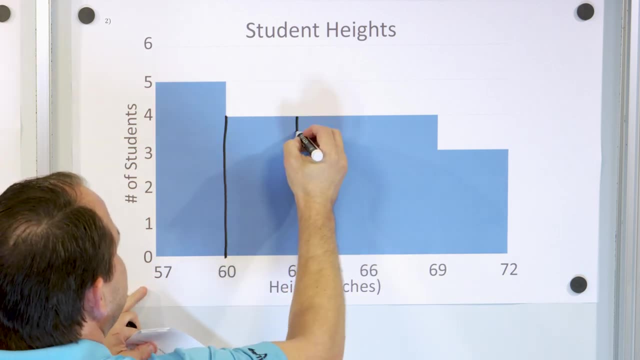 Now, in my particular program I don't have any. everything's pushed together, but I don't have any gaps, So it's a little hard to read. So if you want to, you can draw lines. Some people like to see these lines, some people don't. You can do whatever you want To me. I'm not a real stickler, I just want you to be able to read the thing. 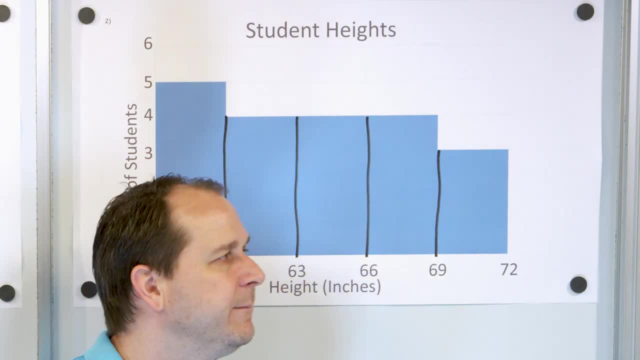 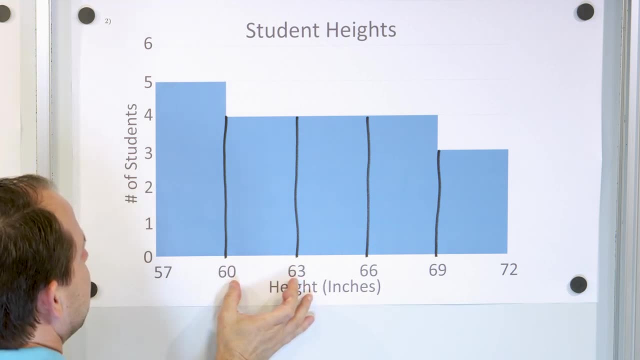 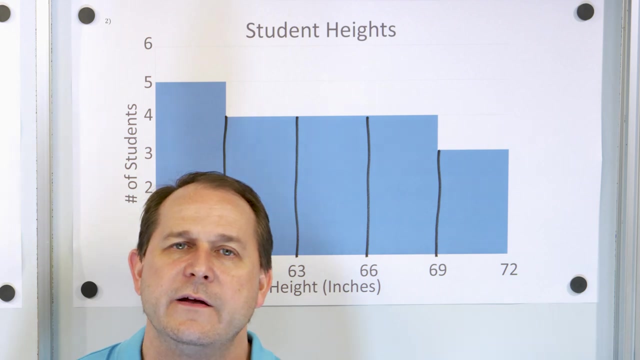 But you should not have any gaps between them, all right. So the question is: how do we read this thing So you could say, for instance, between 60 and 63 inches. right, We had four students in there. Now it doesn't tell me the actual heights of those four students. So a histogram. it's taking the data you have and it's presenting it to you without showing you every single data point. 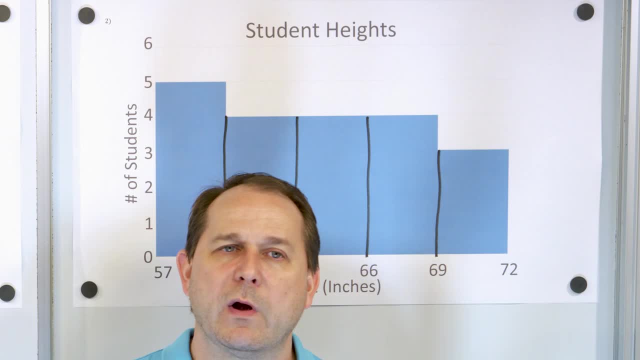 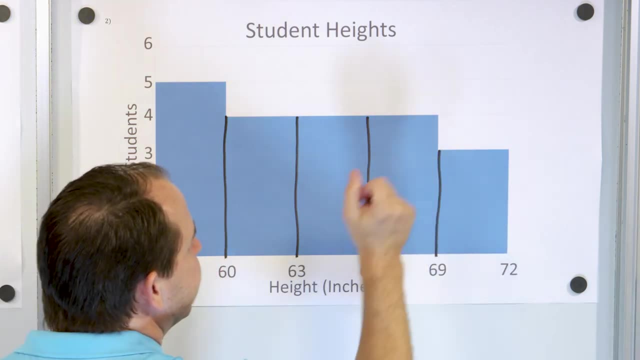 We are throwing some data away because we want to get an overall picture of what's happening And you can look at this And say, well, OK, I have most students down in this range and I have the least number of students over in this range. 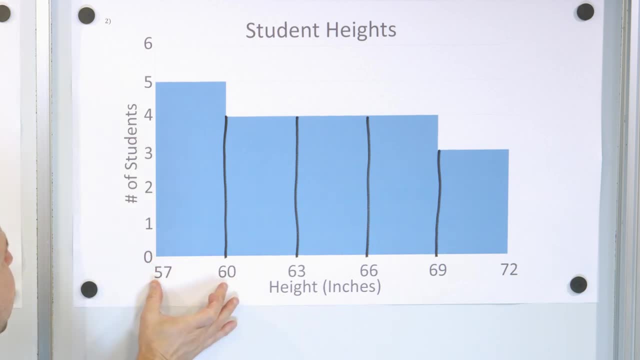 But we lose a little bit of the raw data because we only know, for instance, between here, between 57 and 60 inches. we had five students, But I don't know if they were 58 inches or 57 inches or 59.. 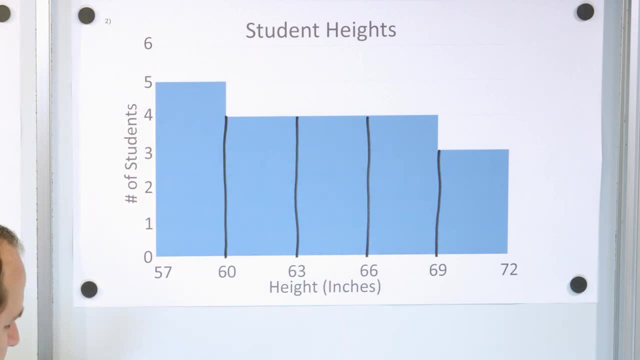 I don't really know. I just know I have five of them in this window. All right, let's take a look at question number one. All right. question number one says how many students are 66 inches or taller. How many students are 66 inches or taller? 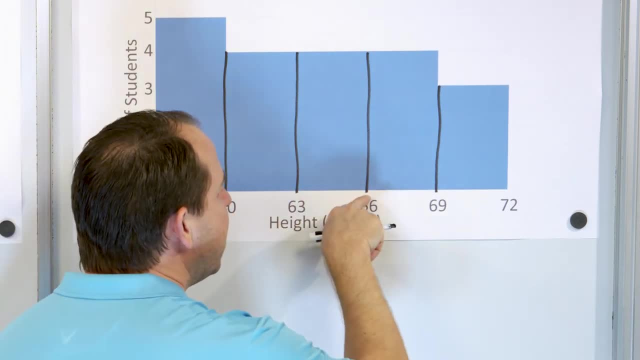 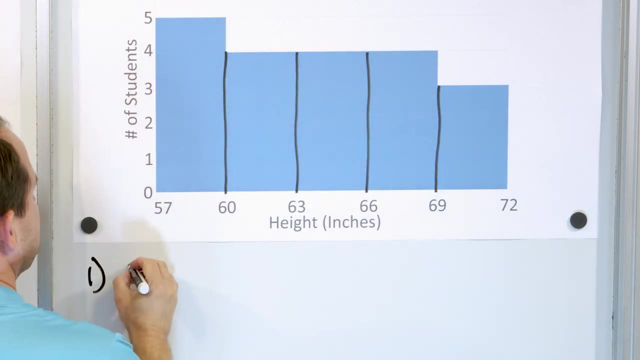 So I look down here at the height in inches, I go to 66 inches And anything taller than that would be all the way to the end of the chart. So I know, from 66 to 69, I have four, And I know that I have another window from 69 to 72 inches. 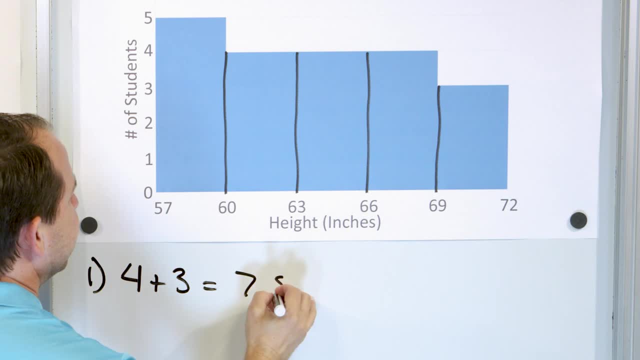 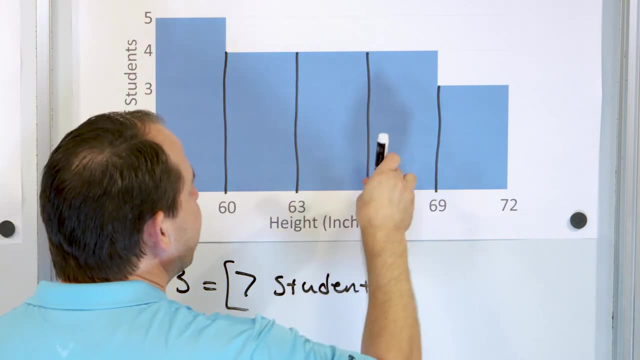 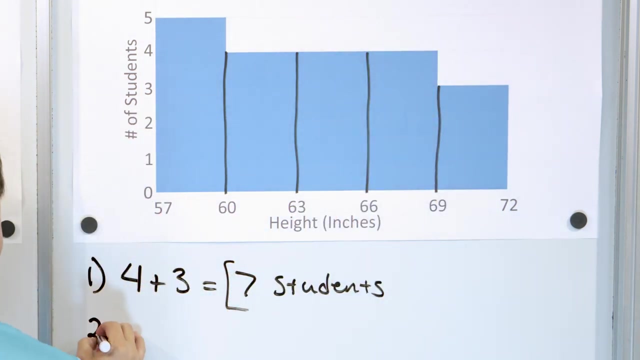 I have three more students that height. So the answer is seven students, because the question asked how many students are 66 inches or taller. So it's basically looking at The chart and adding everything up to the right: This many students plus this many students. 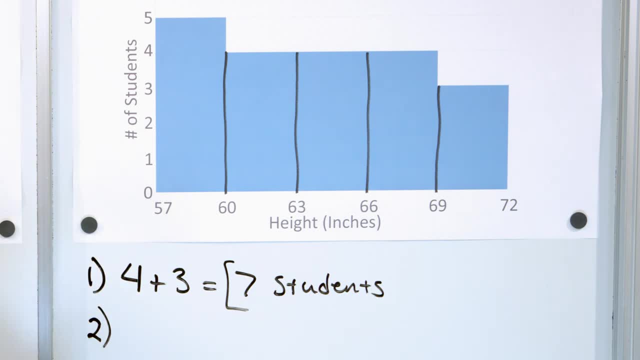 Problem number two: how many students are between 60 and 66 inches taller? Well, here is 60 and here is 66 inches, So it's like two bins here, And we know that between 60 and 63 is four and between 63 and 66 is another four. 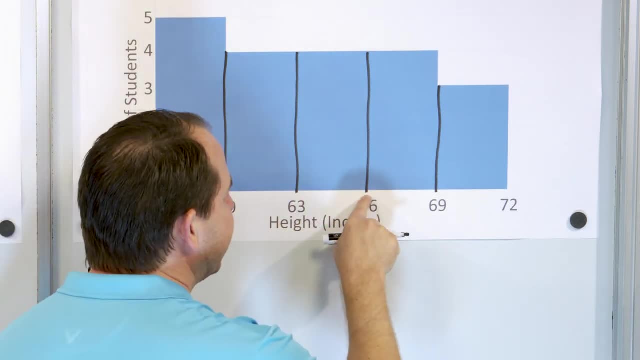 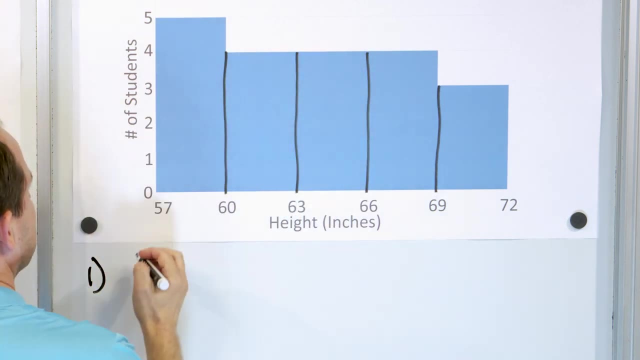 taller. So I look down here at the heighted inches, I go to 66 inches and anything taller than that would be all the way to the end of the chart. So I know from 66 to 69, I have four And I know that. 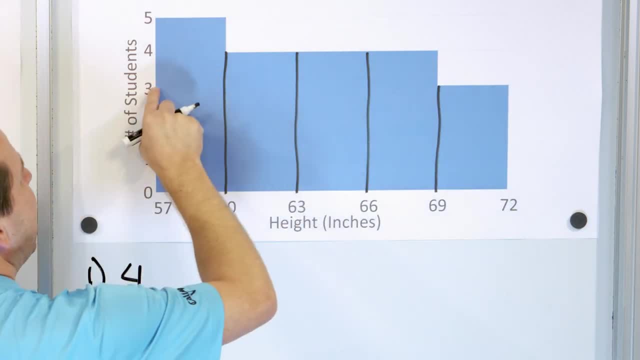 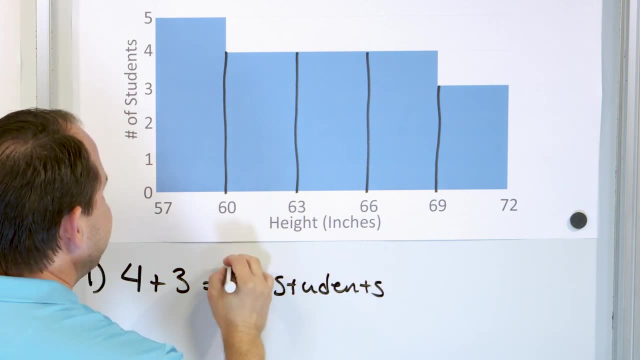 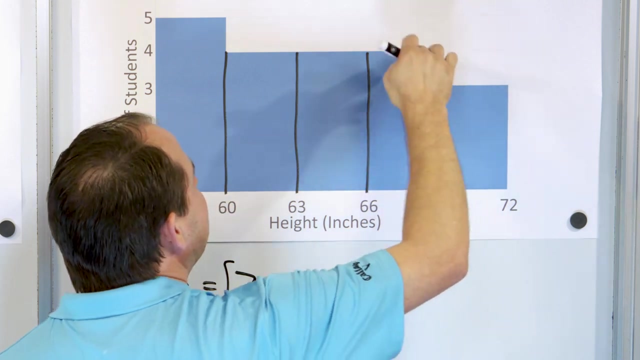 I have another window from 69 to 72 inches. I have three more students that height, So the answer is seven students, Because the question asked how many students are 66 inches or taller. So it's basically looking at the chart and adding everything up to the right: This many students plus this many students. 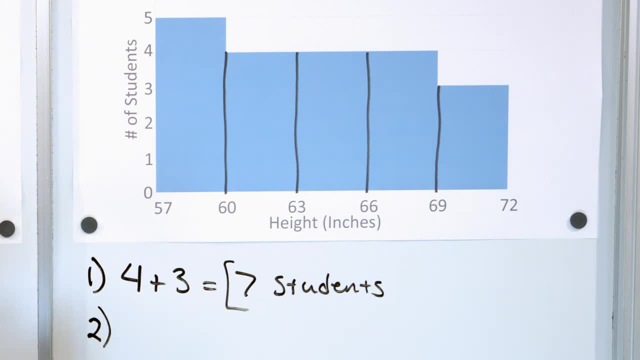 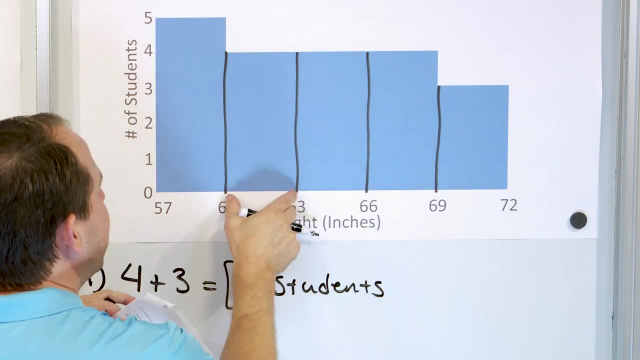 Problem number two: how many students are between 60 and 66 inches taller? Well, here is 60 and here is 66 inches, So it's like two bins here, And we know that between 60 and 63 is four, and between: 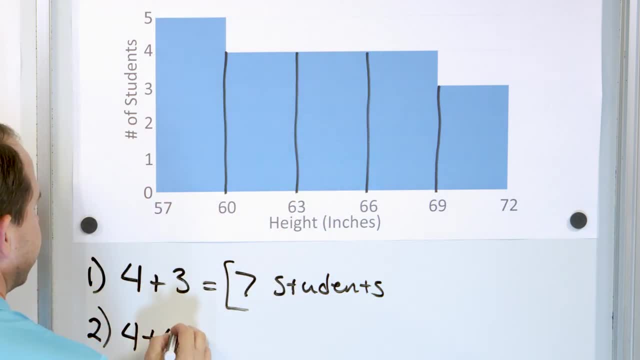 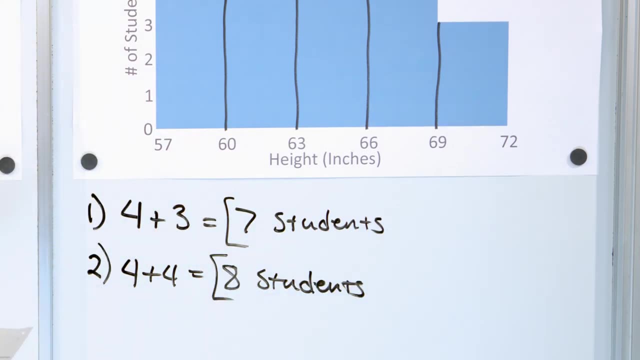 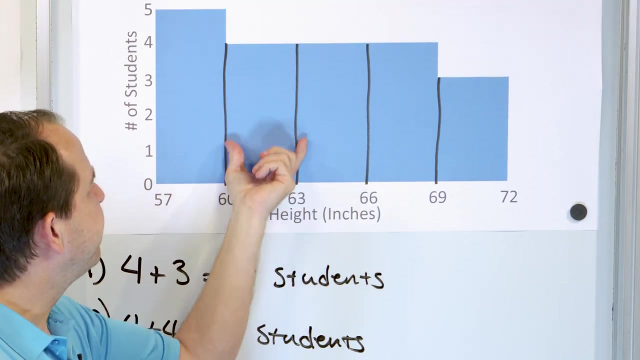 63 and 66 is another four, So you have to add those together Eight students. So the question was how many students are between 60 and 66 inches? We have to take a look at two adjacent bins that are next to each other and add up the results. So when people look at histograms, 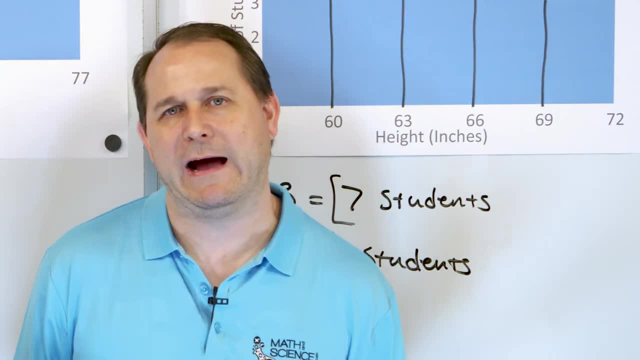 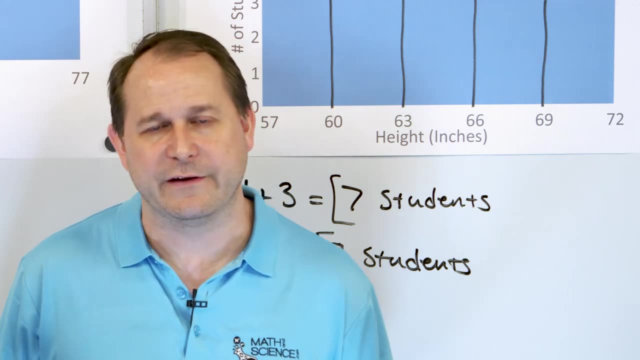 the first thing they say is: oh, it's a bar graph. And essentially it is a bar graph. A lot of books and teachers tell you: oh, it's so much more complicated. It's really not complicated. It does look like a bar graph. The main differences are: when you draw a bar graph, those bars usually. 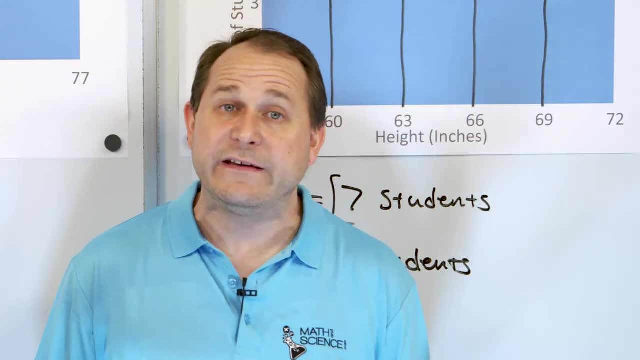 have a bar graph. So when you draw a bar graph, those bars usually have a bar graph. So when you draw a bar graph, those bars usually have a bar graph. So when you draw a bar graph, those bars usually have gaps between them. But we never have gaps in a histogram, And the reason we don't have gaps 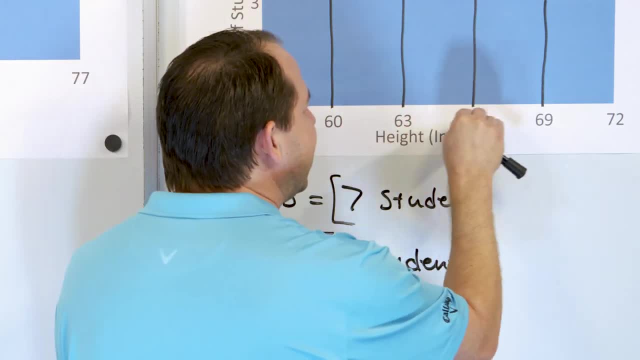 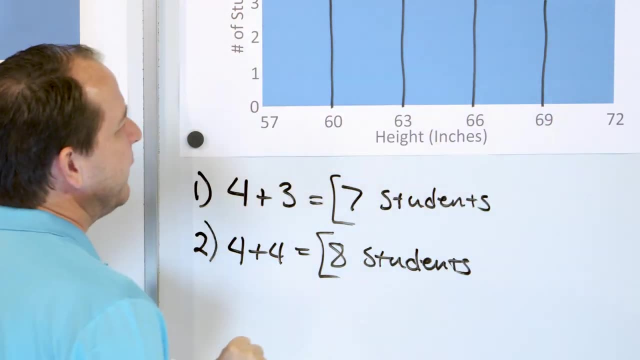 by the way, is because the numbers along the bottom are not labels, like you know. do you like apple pie or blueberry pie, or you know pecan pie or whatever? We don't use words along the bottom like we do for a bar graph. We have numbers, But not only that. we have windows. We call them bins. 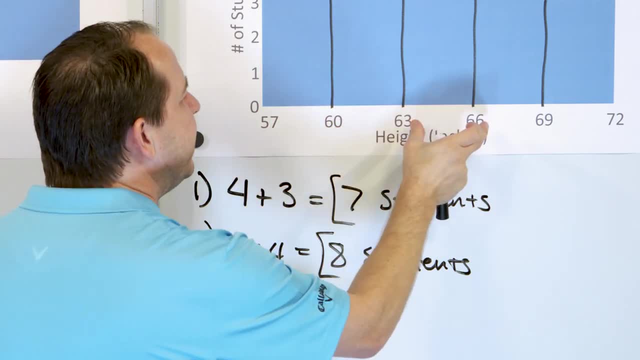 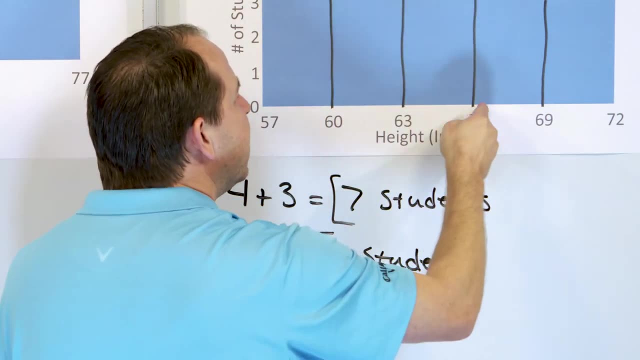 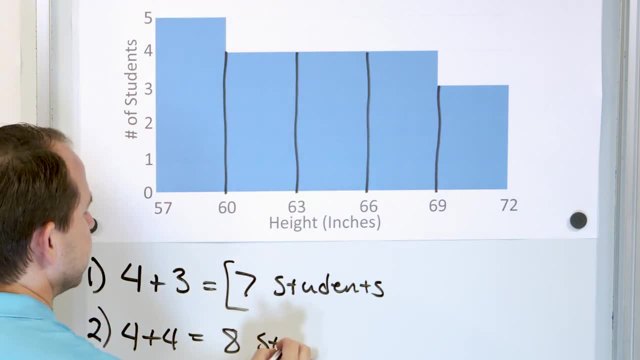 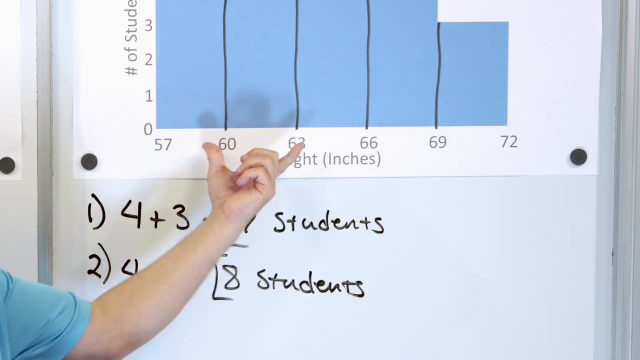 So you have to add those together: Eight students, Right? So the question was: how many Students are between 60 and 66 inches? We have to take a look at two adjacent bins that are next to each other and add up the results. 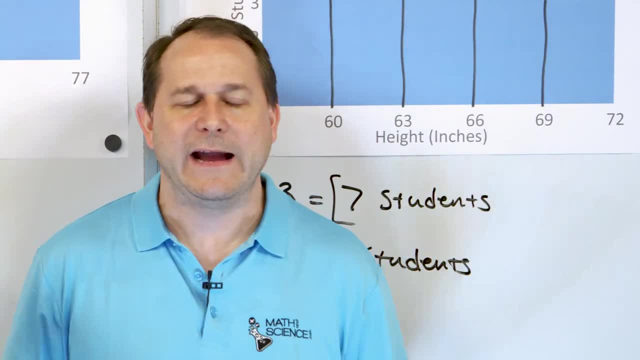 So when people look at histograms, the first thing they say is, oh, it's a bar graph. And essentially it is a bar graph. A lot of books and teachers tell you: oh, it's so much more complicated, It's really not complicated. 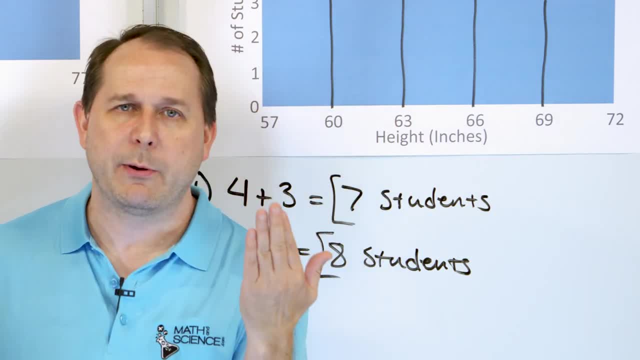 It does look like a bar graph. The main differences are: when you draw a bar graph, Those bars usually have gaps between them, but we never have gaps in a histogram, And the reason we don't have gaps, by the way, is: 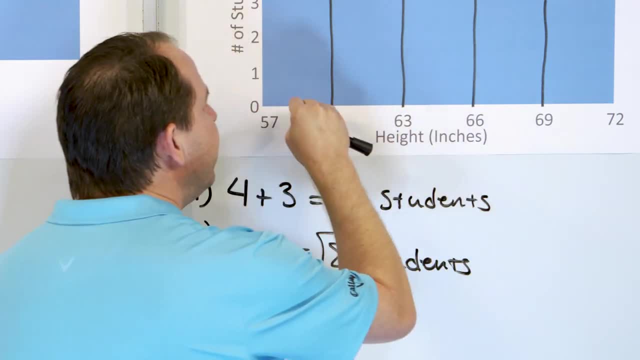 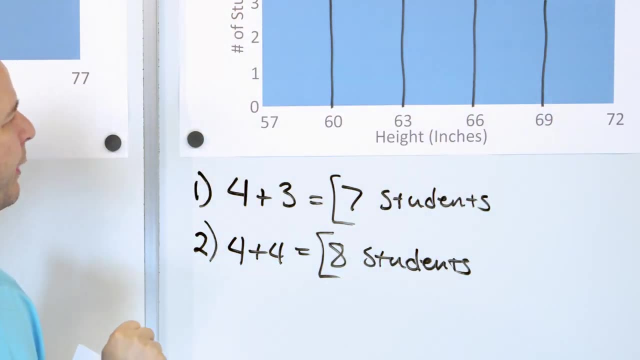 Is because the numbers along the bottom are not labels. like you know, do you like apple pie or blueberry pie, or you know pecan pie or whatever? we don't use words along the bottom like we do for a bar graph. We have numbers. 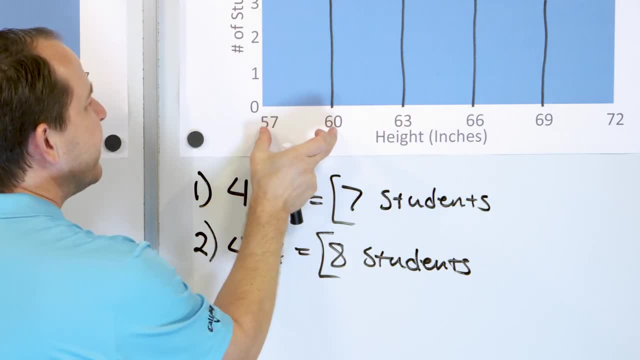 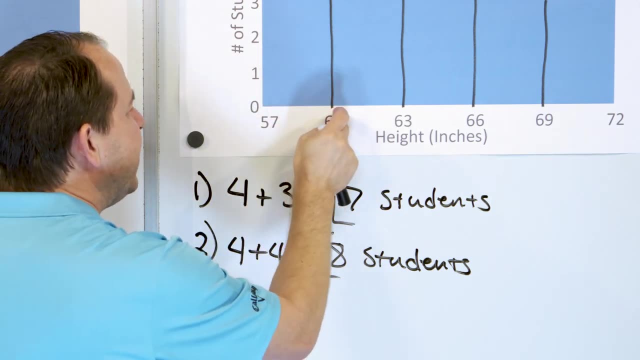 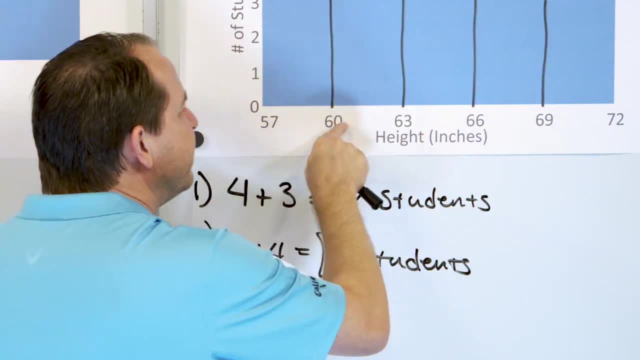 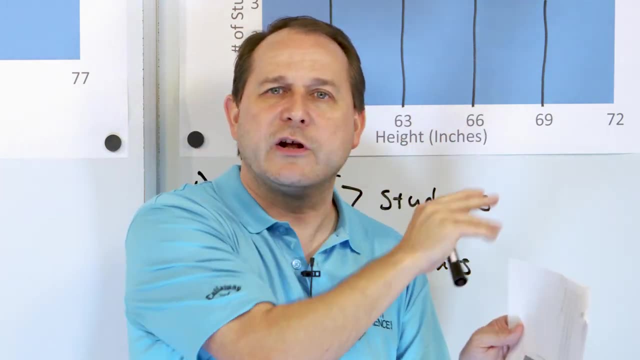 And that's why there's no space between them. We want to push them all together Because this number, these numbers- we don't want any gaps between the numbers- is the bottom line, So we want to push them all together, put numbers along the bottom with the same width of bins. 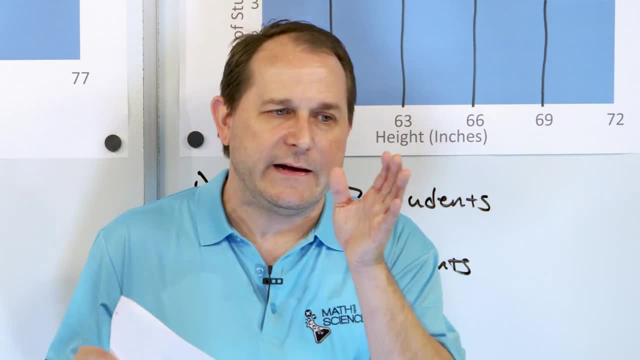 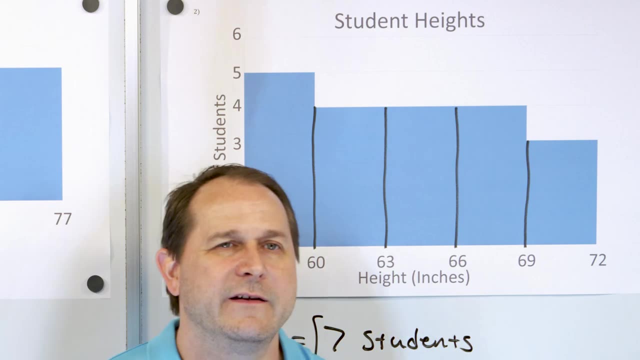 And then we're just counting the number of times that it happens in each of those bins. So we're counting the number of students in this window and the number of students in this window, and so on. So that's another way of saying we're measuring the frequency. 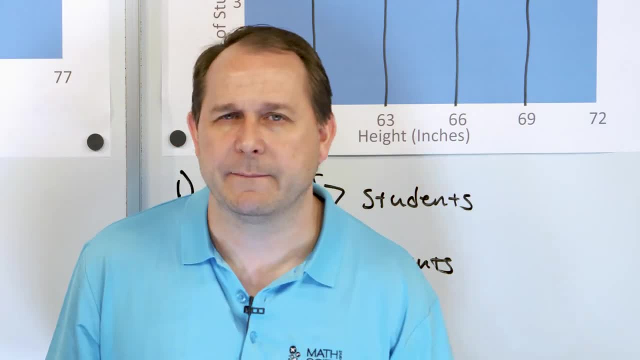 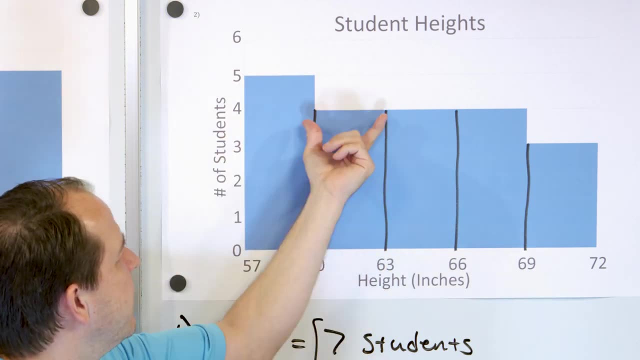 Frequency is a fancy word. Frequency just means the number of times something happens. So the number of times, So the number of students this window happens is five. The number of times or students that we have between these heights is four, and so on. 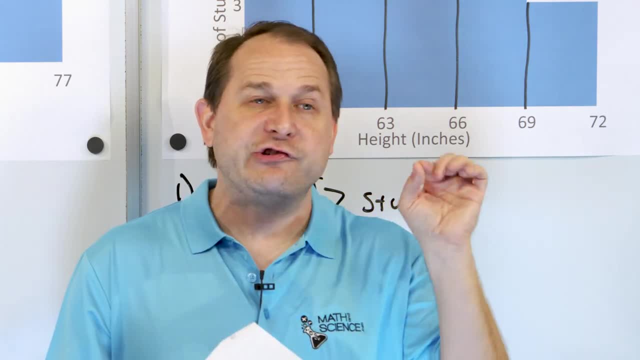 It's kind of a way to talk about it in a little bit different way. We're not showing all the data points, We're just counting how many times something happens. That's the main difference. So I'd like you to go through this. 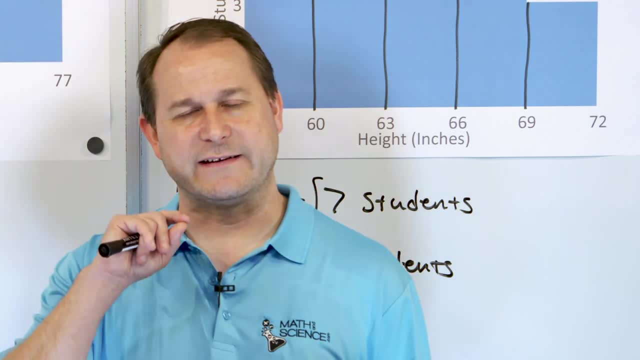 Make sure you understand what a histogram is and how to use it. Follow me on to the next lesson. We're going to continue learning about histograms.